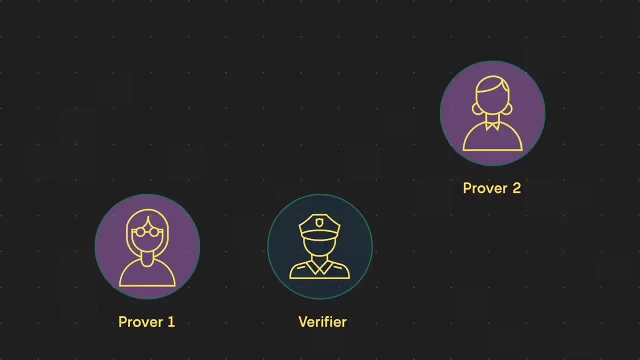 and confirm every single detail of the suspect's stories. but by asking the right questions and pitting your subjects against each other, you can catch them in a lie or develop confidence that the facts check out. The policemen will place these two suspects in different rooms, but it just so happens. 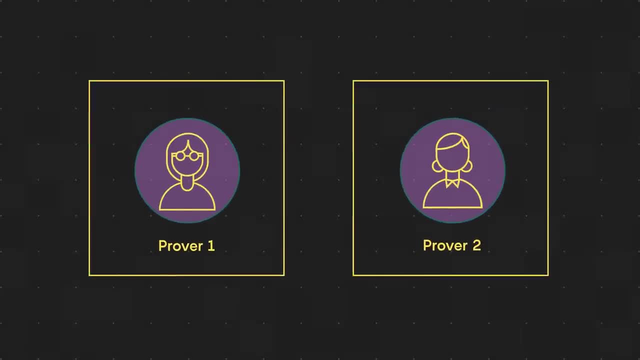 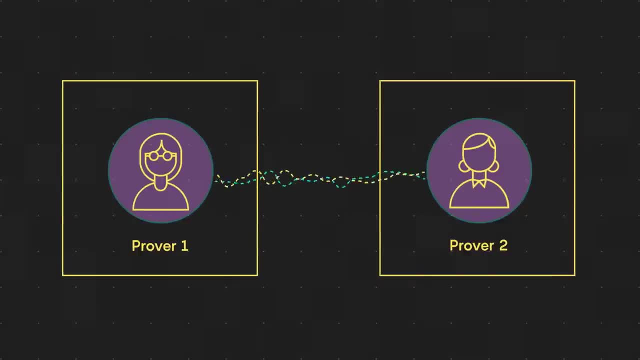 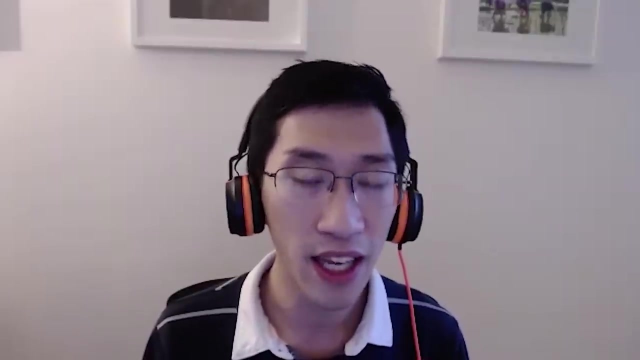 to coordinate their responses in some spooky quantum mechanical fashion. The policeman's job is to try to figure out what the truth really is. The main result of this paper is that, even though the suspects might share quantum entanglement, the policemen can actually interrogate them in such a way that the policemen can figure. 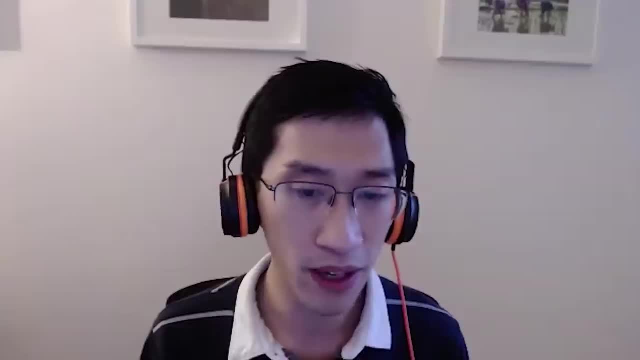 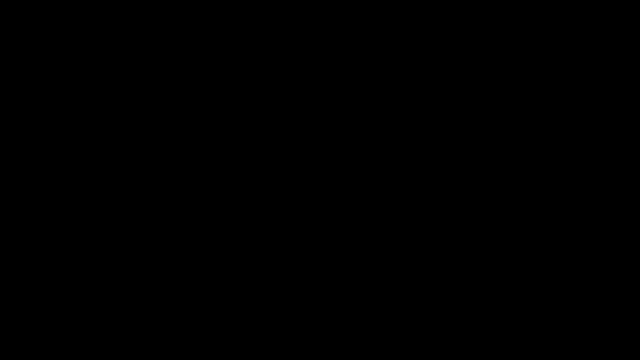 out the truth of any mathematical statement corresponding to an enormously nuanced and complex mystery. Those are the two possibilities. It's very complicated to explore the truth. complicated range of questions. This means that in theory, a super powerful quantum computer could verify answers to even unsolvable problems. 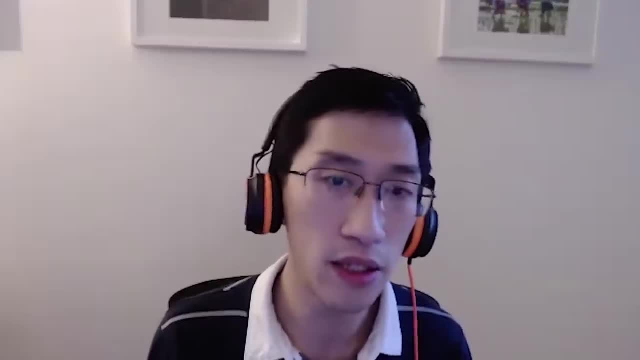 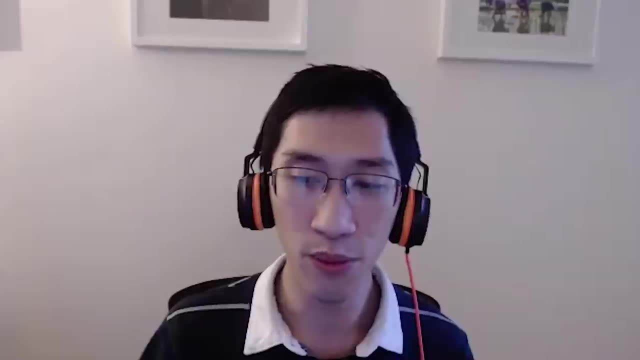 like Turing's halting problem. It involves all these really beautiful pieces from different areas, things from computer science, things from mathematics and physics that before we didn't think were that related to each other, and yet they are. I think it points to something much more interesting. 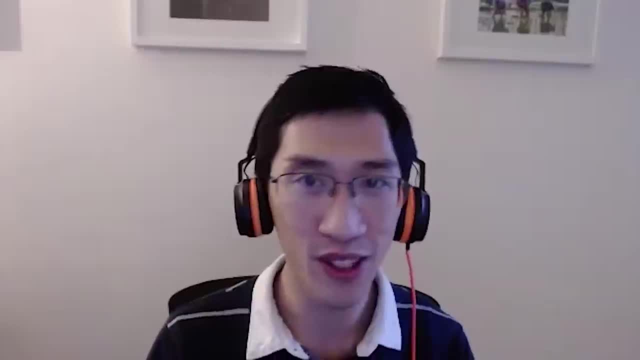 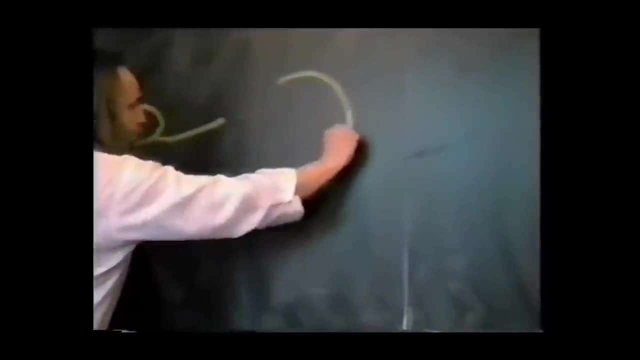 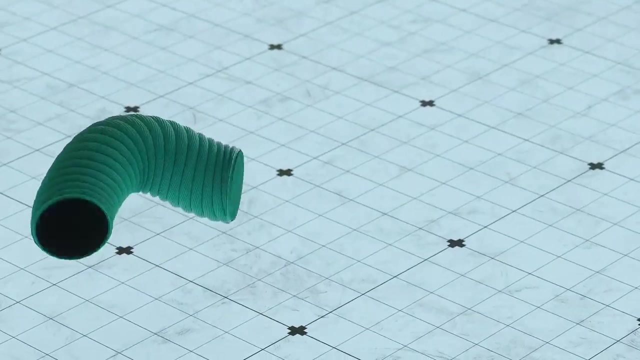 I don't know what, but there's a feeling that there's something more to you know. there's like a whole new world to discover. This is John Horton Conway. His infamous knot problem eluded mathematicians for half a century. The question asked whether 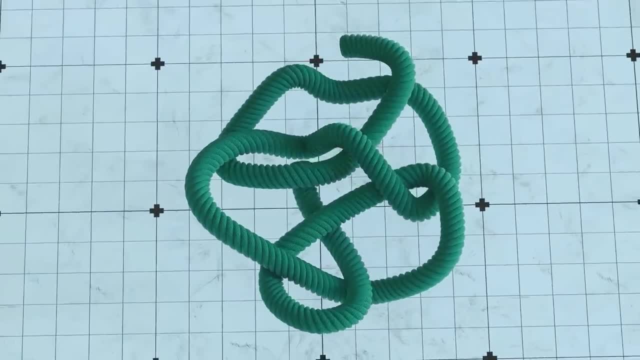 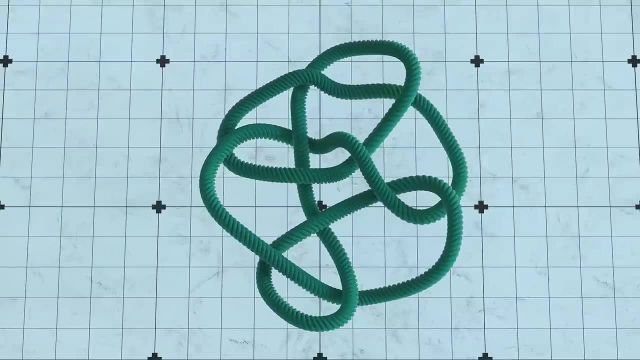 the Conway knot was actually a slice of a higher dimensional knot, a property called sliceness. This question proved answerable for thousands of similar knots, but Conway's resisted every attempt to untangle it. Lisa Piccirillo was a graduate student when she first. 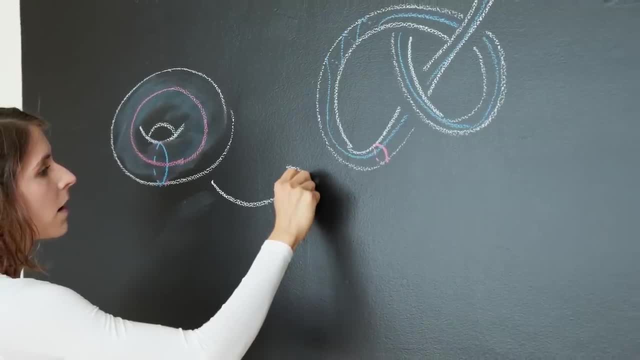 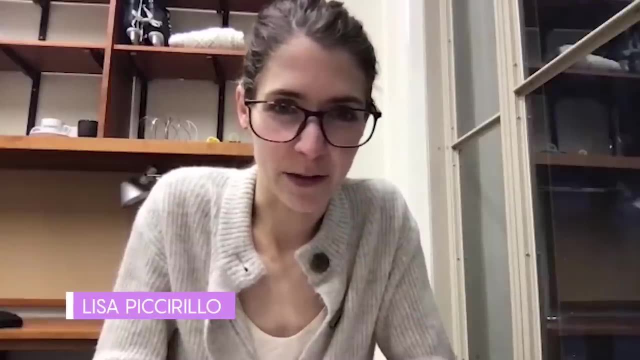 heard about the Conway knot. Well, I just thought it was completely ridiculous that we didn't know whether this knot was sliced or not. We have a lot of tools for doing this sort of thing, so I didn't understand why, for some 11 crossing knot, this should. 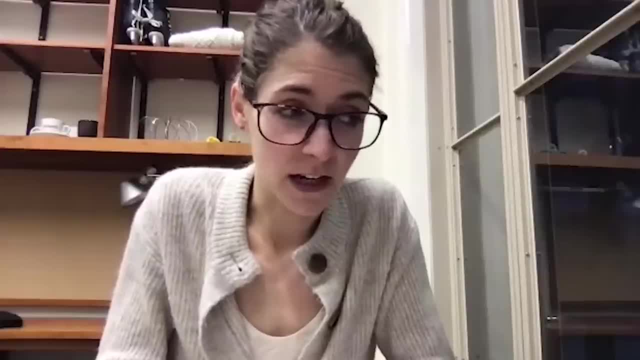 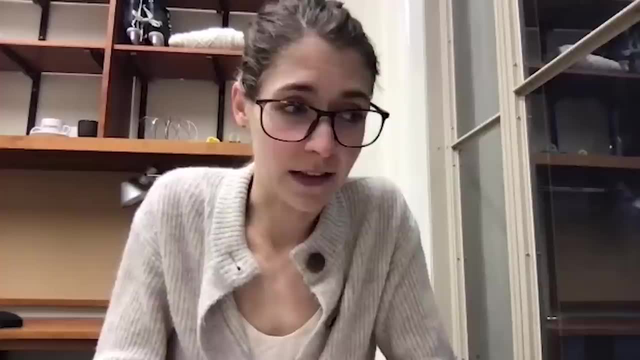 be so difficult. I think the next day, which was a Sunday, I just started trying to run the approach for fun and I worked on it a bit in the evenings, just to try to see what's supposed to be so hard about this problem. 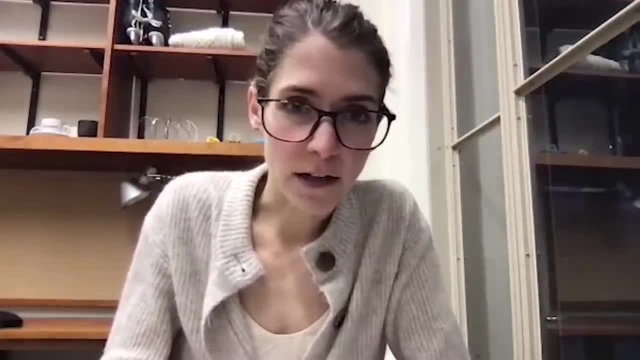 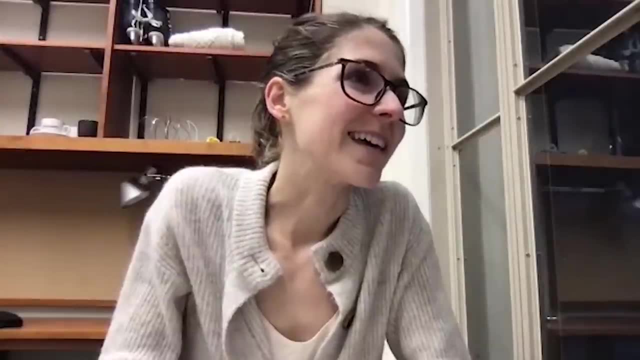 And then the following week I had a meeting with Cameron Gordon, a senior topologist in my department, about something else and I mentioned it to him there. He was like: oh really, You showed the Conway knot's knot slice, Like, show me. 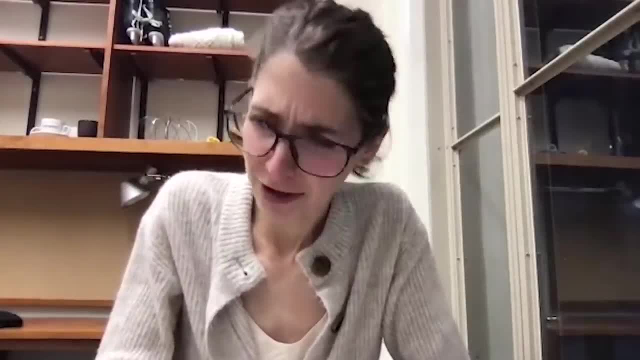 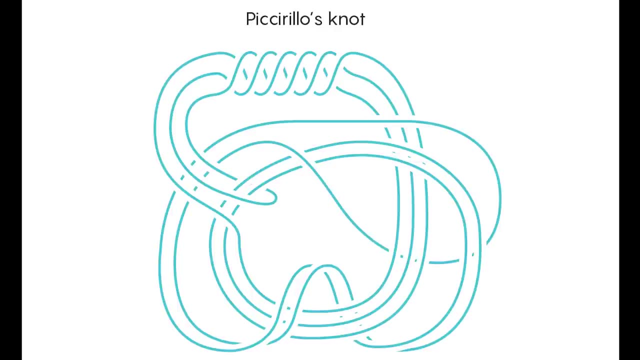 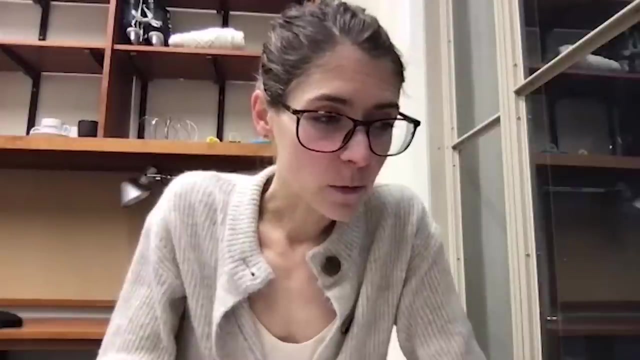 And then I started to put it up and he started asking kind of detailed questions and then at some point he got very excited. Piccirillo's proof was published in the Annals of Mathematics. It was quite surprising to me. I mean, it's just one. 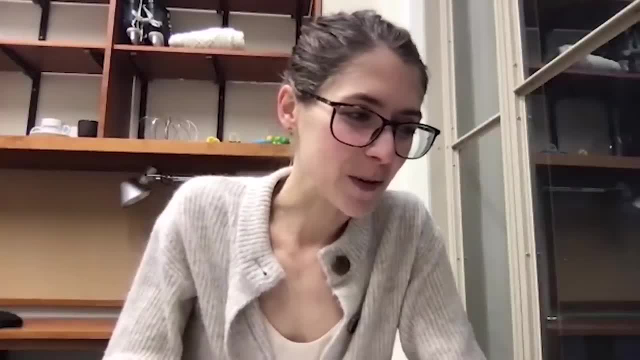 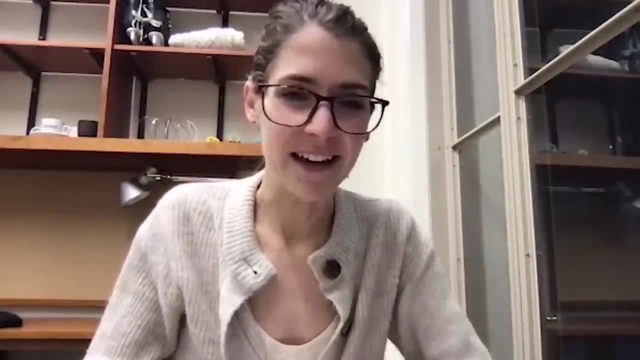 knot. In general, when mathematicians prove things, we like to prove really broad general statements. All objects like this have some property and I've proved like one knot has a thing. I don't care about knots, So I do care. 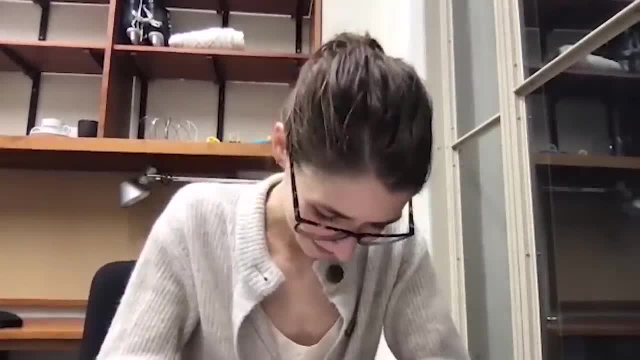 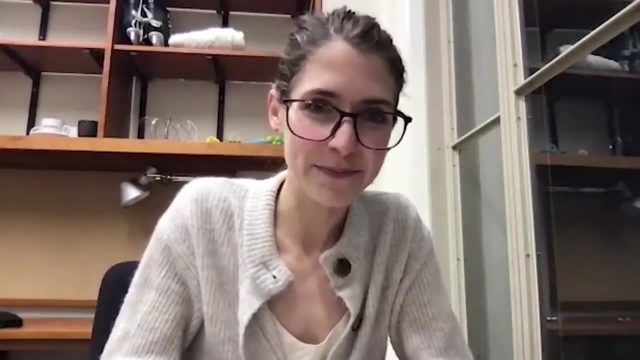 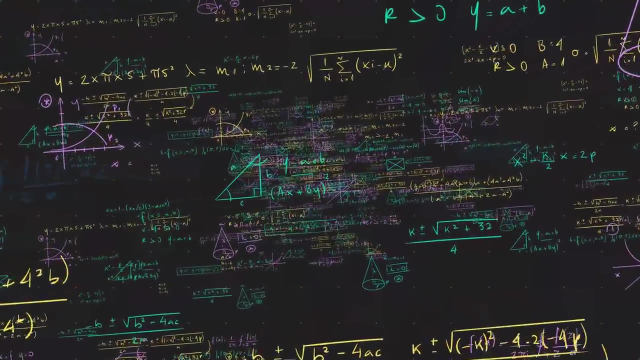 about three- and four-dimensional spaces, though, And it turns out that when you want to study three- and four-dimensional spaces, you find yourself studying knots anyway. Mathematics can sometimes seem like a jumbled mosaic. Major areas of study have never been fully. 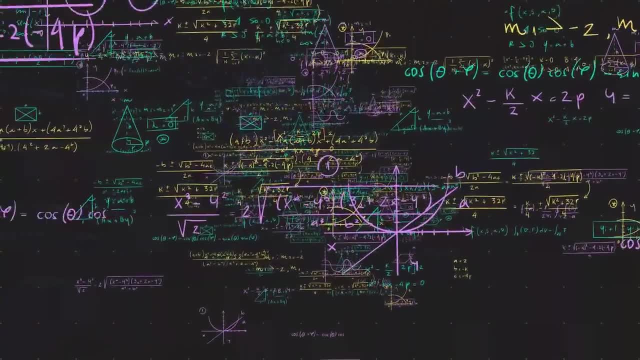 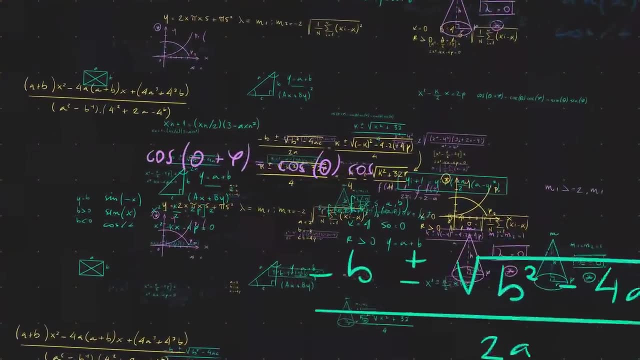 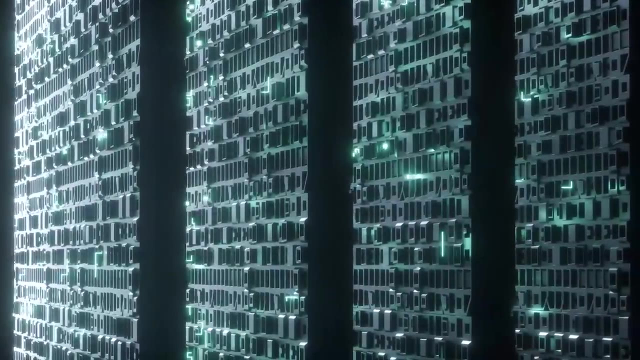 written down, and doing so would have required using thousands of other definitions that don't yet exist. Now imagine you had a library of Alexandria that contained the entire history and the sum total of mathematical knowledge. With everything cataloged, you could program an AI to verify increasingly complex 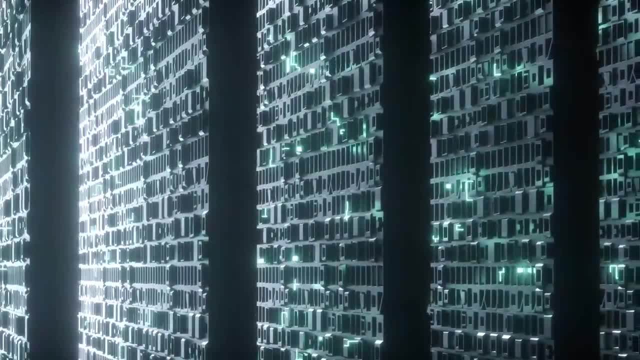 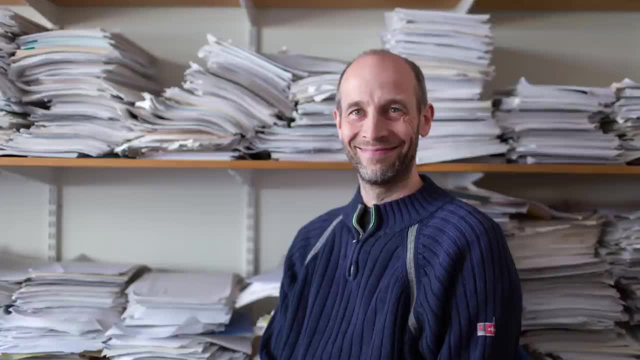 proofs and one day, hopefully, come up with new ones on its own. At Imperial College London, Kevin Buzzard is in the process of digitizing math. He's teaching it to a software called Lean, which draws upon an ever-growing library. 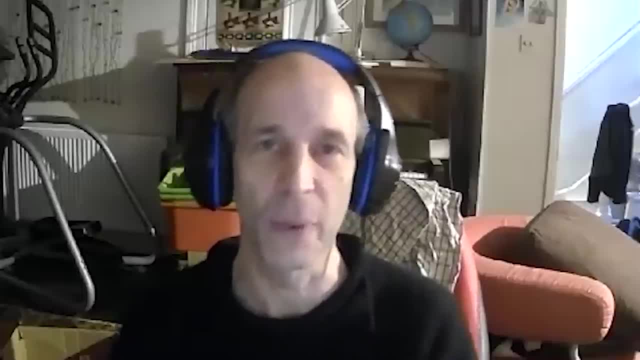 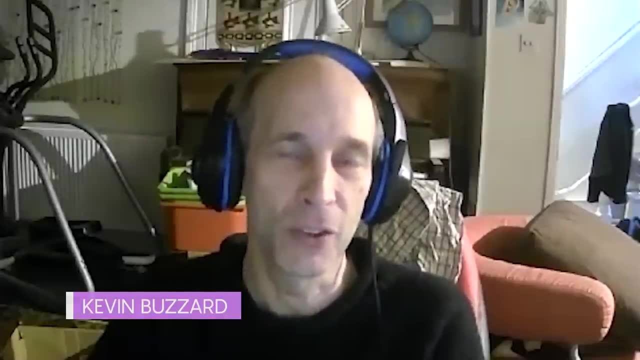 of proofs and theorems. I decided that this software was very interesting about three years ago and I've since made a huge amount of noise about it. We took some very, very modern mathematics and just showed you know, we taught it to Lean and Lean could handle it. 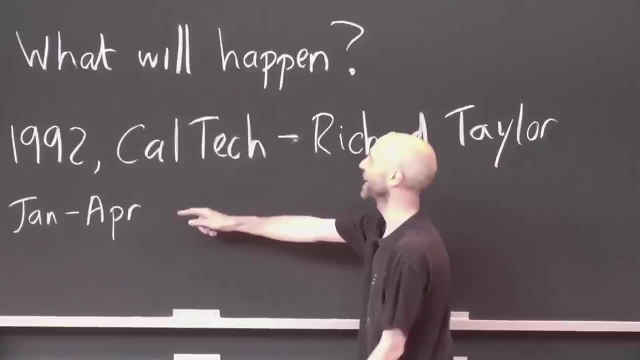 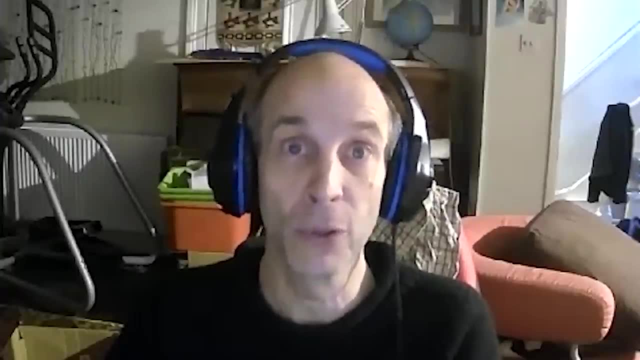 And basically it was at that point that I realized it should be able to do anything really. Lean has a big maths library, 450,000 lines of code long. The library just grows all the time. Every day, you know, 10 more pull requests.